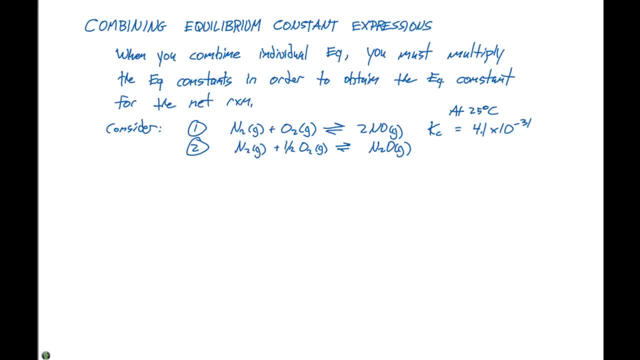 N2O gas, our Kc is equal to 2.4 times 10 to the minus 18.. So what is the Kc at 25 degrees Celsius for the following reaction: N2O as a gas plus 1 half O2 gas in. 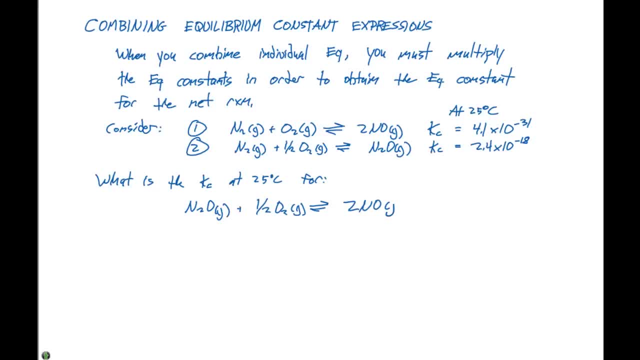 equilibrium with 2NO gas. So we have to figure out how to first of all come up with this overall equation. So if we look here, N2O shows up as a reactant in our case, here that we're solving for, and 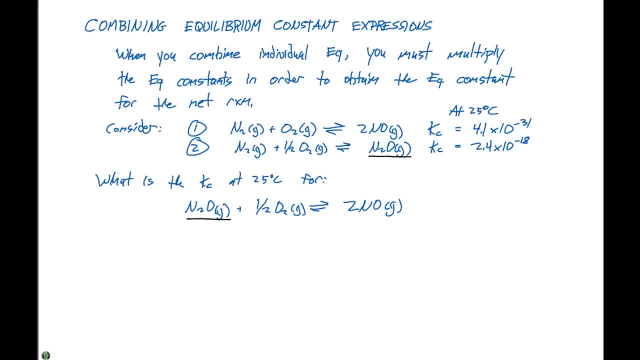 as a product in an initial set of reactions. The O2 gas shows up here and in two places up here. The NO gas shows up here and also shows up here. both as a product only shows up in these first two equations, right here. 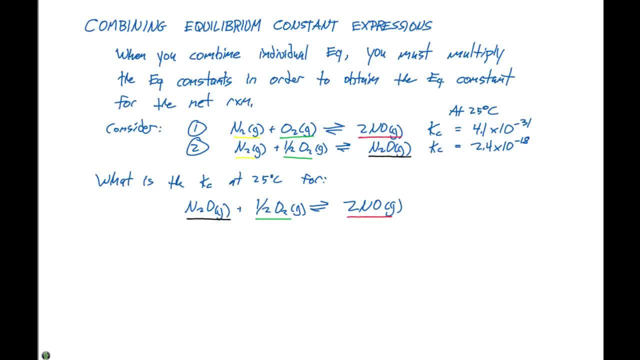 And that indicates to us that it will be an intermediate. So in order to get each of these here, we're gonna need to do two things: We're gonna have to reverse reaction number two and we're gonna have to use then reaction number one and add them together. 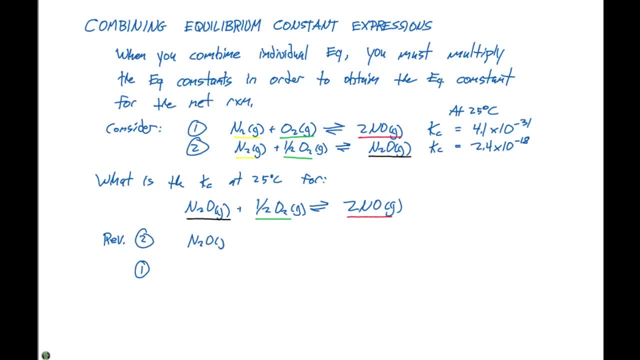 So if we reverse reaction number two, that gives us N2O gas in equilibrium with N2 gas plus a half O2 gas, The Kc for this expression is going to be 1 over 2.4 times 10 to the minus 18.. 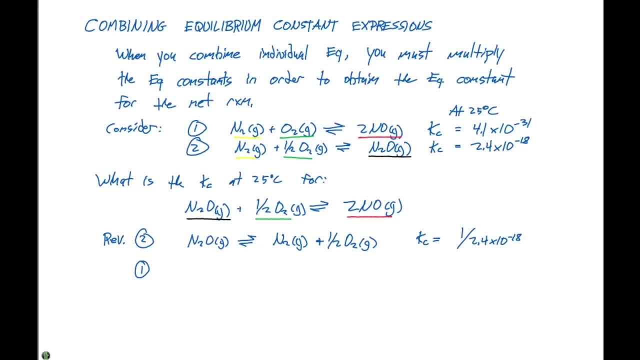 Cuz remember, when we reverse a reaction, we need to do the reciprocal. The first reaction then is gonna be N2O, N2 gas plus O2 gas in equilibrium with 2NO gas, So the Kc of this is going to be 4.1 times 10, to the minus 31,. 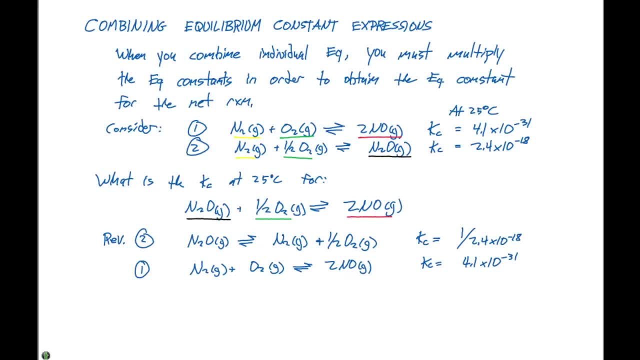 which is what we have here. Now. we need to add these two together. The nitrogens are gonna cancel out. We have N2O gas over here. on the left hand side, we also have an O2 gas, but we have a half of one over here. 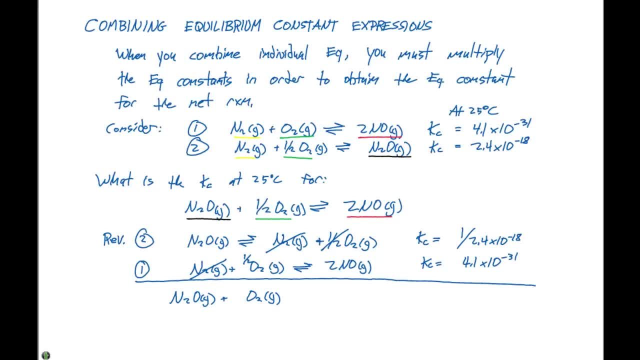 So this is gonna cancel out with that and we're gonna have a half left over here. So we have N2O plus a half O2 in equilibrium with 2NO gas, which is what we're asked for, and now we have to figure out what the Kc of this is. 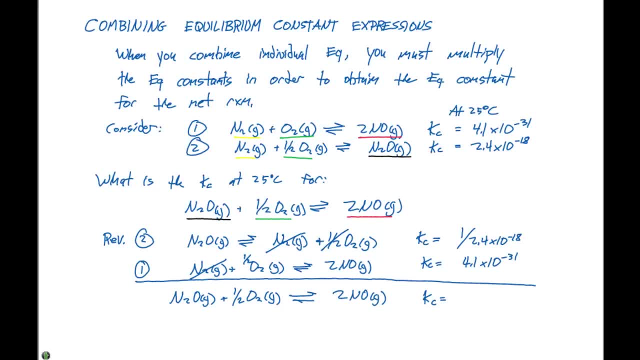 So if we're determining an equilibrium constant for a net reaction that's made up of two or more reactions, The Kc, or the equilibrium constant, is going to be the product of all of these equilibrium constants, So it's gonna be 1 divided by 2.4 times. 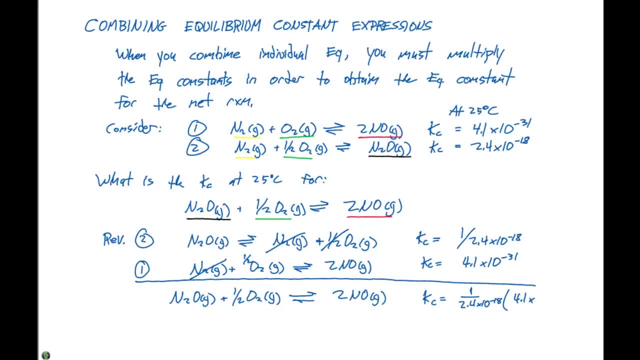 10 to the minus 18 times 4.1 times 10 to the minus 31.. When we go through and multiply these out, our general properties of C and A are going to be: O water, M, water naught, minus CGO. 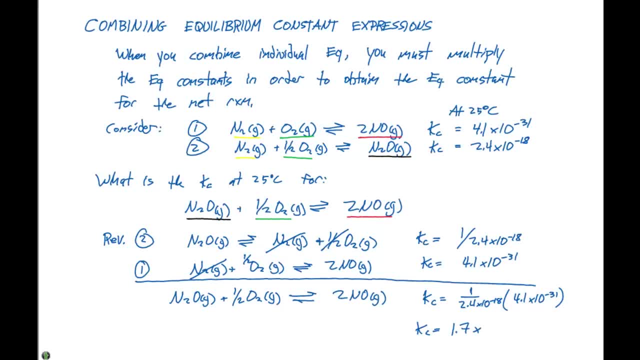 our Kc is gonna equal 1.7 times 10 to the minus 13. And this is gonna indicate that this will not go forward very far and it's gonna favor the reactants. So when you're combining two equations together to get a net reaction, 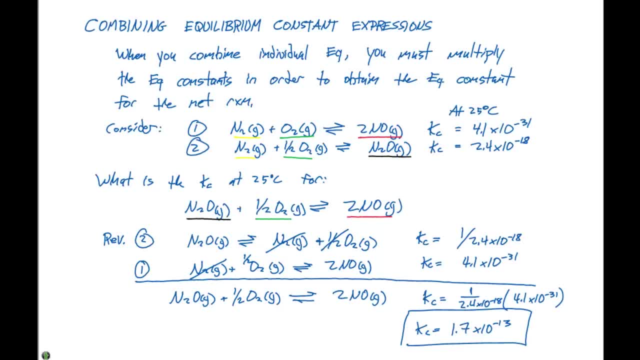 you have to be able to manipulate the steps of that reaction. use the same tactics that we did in the previous video. Then, when we add up all those equations, when we add our two equations here, we're gonna multiply the K values to come up with our overall K for.